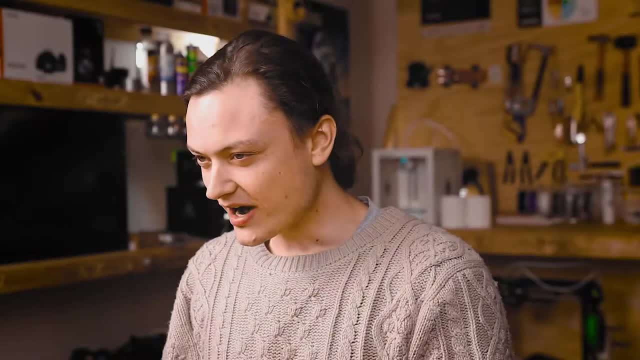 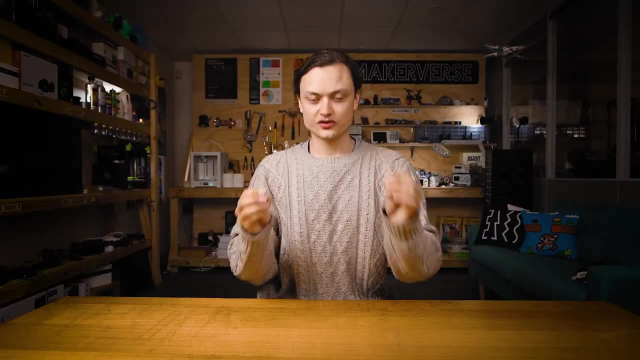 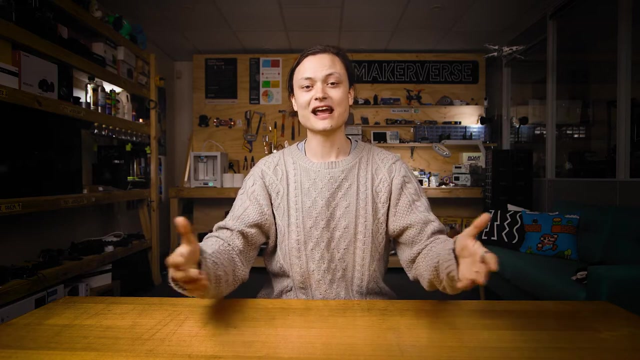 like gamma rays or radiation and x-rays. The radio frequency spectrum, which is what IoT devices and mobile phones work with, sits in the lower part of the spectrum. Spectrum management is the process of regulating the use of radio frequencies with the intent to promote efficient use and 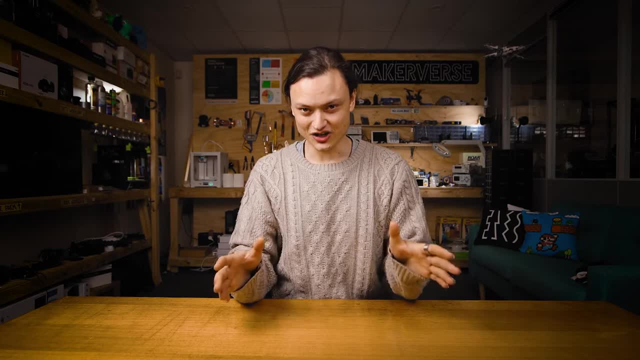 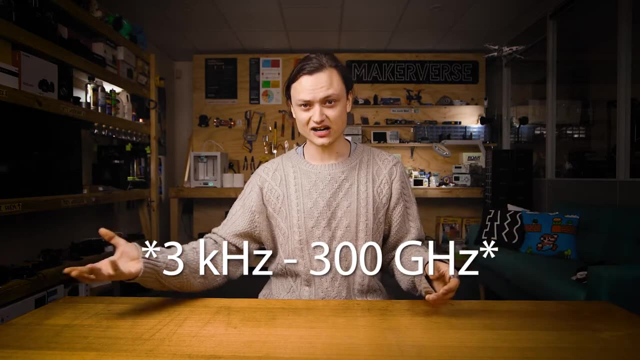 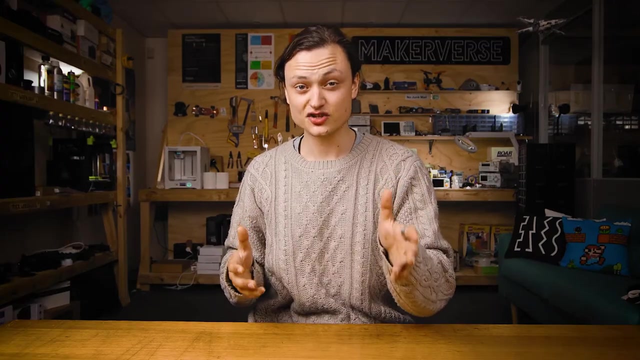 improve society, So maybe now you can see where this is going to go. The term radio spectrum typically refers to the full frequency range from 3GHz all the way to 300GHz, which is just a massive range that may be used for wireless communication, Increasing demand for services such as mobile. 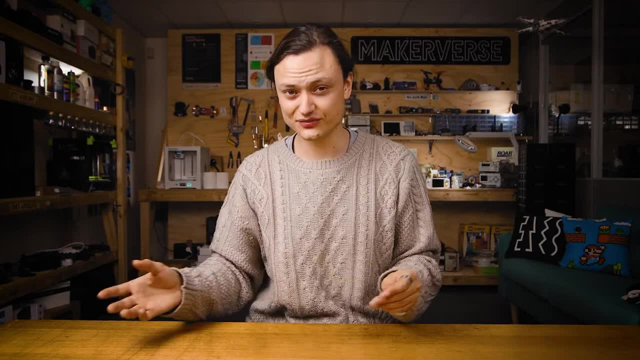 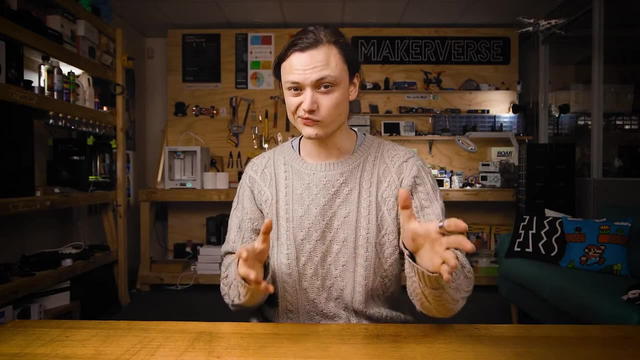 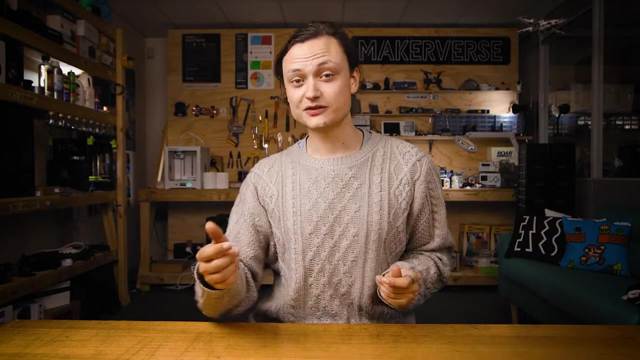 telephones and many others, has required changes in the philosophy of spectrum management, such as. nowadays. there is a massive demand for wireless broadband and the rapid expansion of wireless internet services, And each country has their own different philosophy. Most countries consider the RF spectrum as an exclusive property of the state. The RF spectrum is seen as a national. 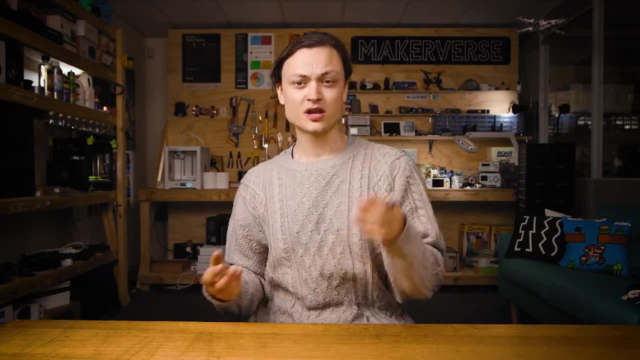 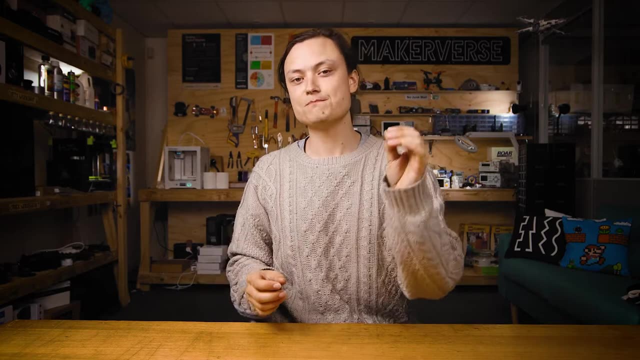 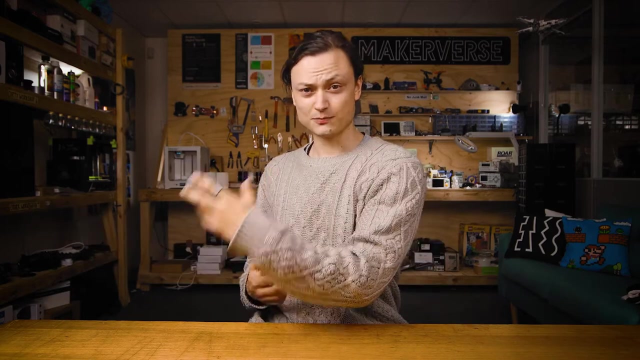 resource. much like water, land gas and more and minerals, RF is reusable. however, unlike those other ones, The purpose nowadays for most of this spectrum management is to mitigate the radio spectrum pollution and maximize the usable radio spectrum. The military, scientific pursuits, space missions, consumers, businesses, airplanes, everyone. 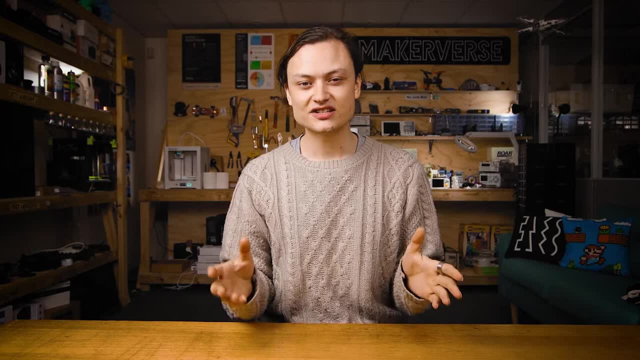 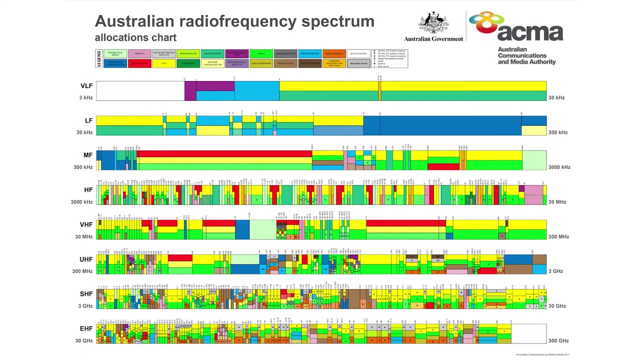 wants a slice of this radio frequency pie, So this landscape becomes very complicated. Now I'll throw up this infograph of the Australian radio frequency spectrum allocation chart just to show the complexity. and this is just for one country. There is a huge amount of factors that further go. 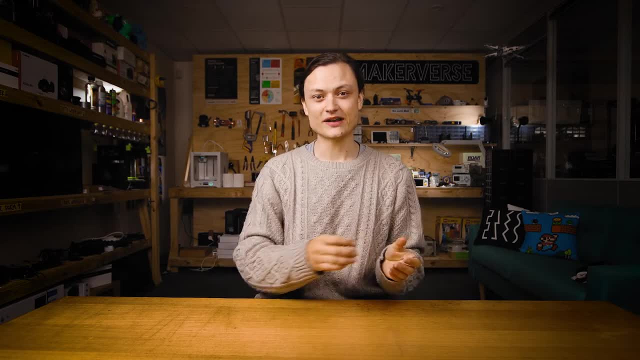 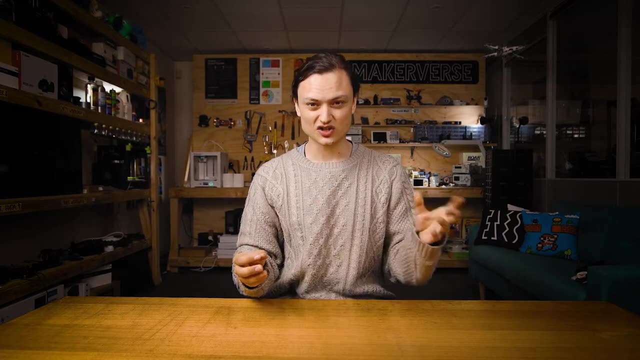 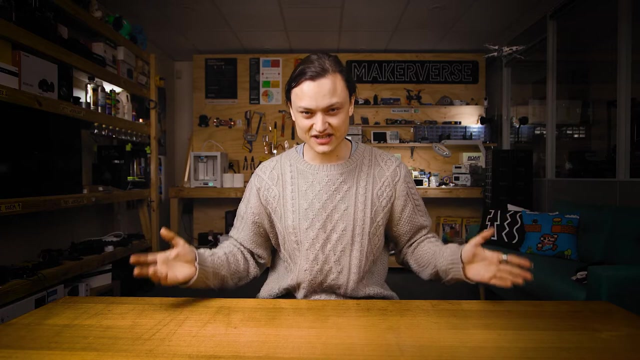 into deciding these allocations, such as the distance the radio wave can travel, whether the wave can penetrate through trees or into buildings, the cost of equipment to transmit and receive, which generally increases as the frequency increases. the longer wavelengths need larger antennas, but they can travel longer distances than short. 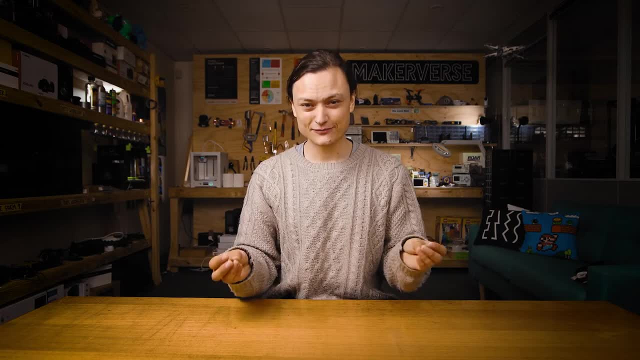 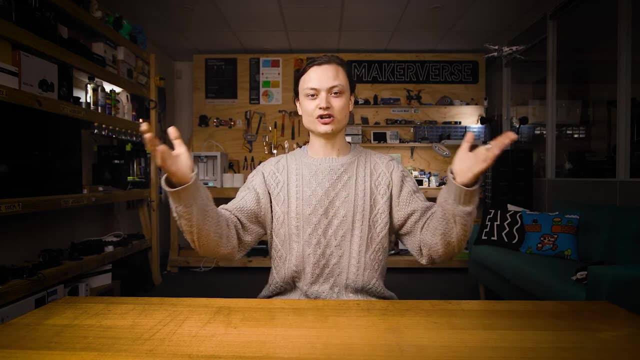 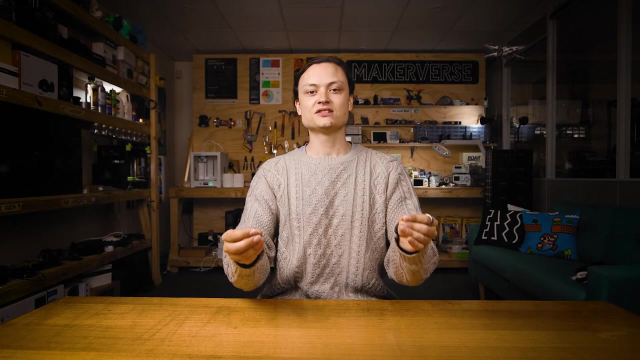 wavelengths and furthermore, different services need different frequencies with different characteristics. So the idea of these organizations, like the Australian Communications and Media Authority, is to match the needs of a service with the right characteristics. This makes for the best use of the spectrum. The result is that some bands are more valuable and in much higher demand than